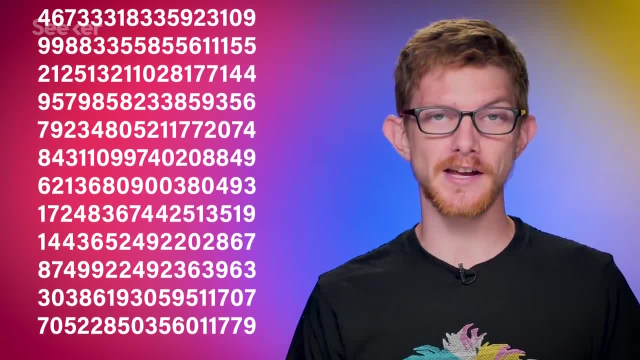 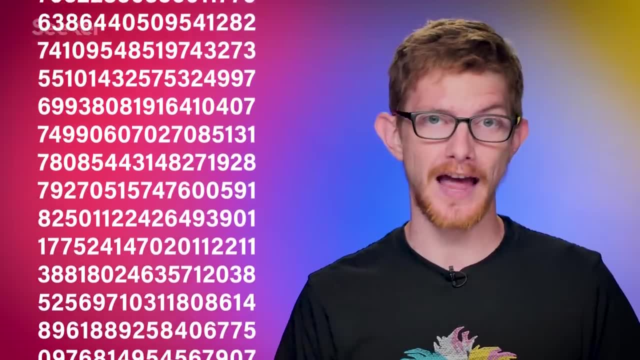 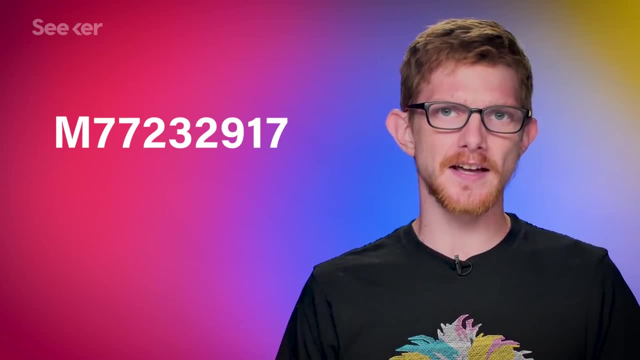 of Germantown, Tennessee. The number is over 23 million digits long, meaning I don't really have time in this video or my entire life, to list the whole thing out, But it's easier to call it by its nickname, M77232917.. It gets its name because that's the exponent. 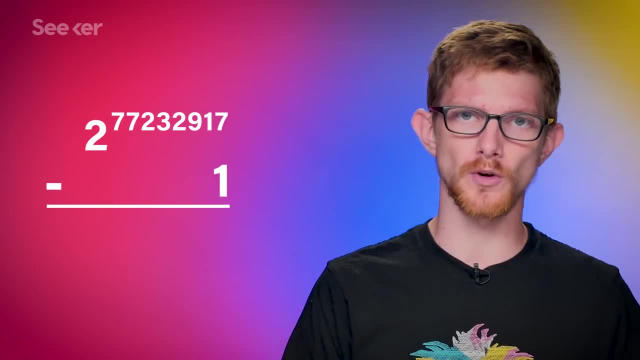 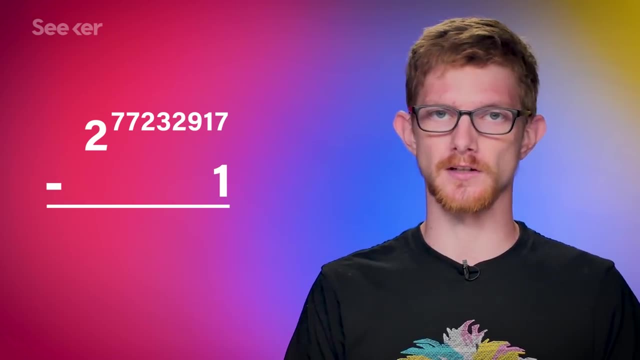 you raise two by to find it. Oh, and don't forget to subtract one when you're done, multiplying 77,232,917 twos together, Otherwise you'll just create a number you can divide by two, and that kind of defeats the whole purpose. 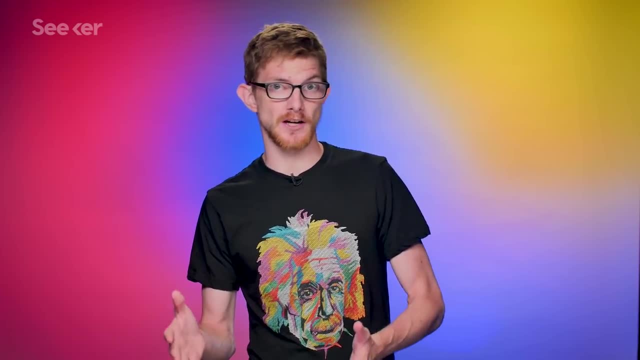 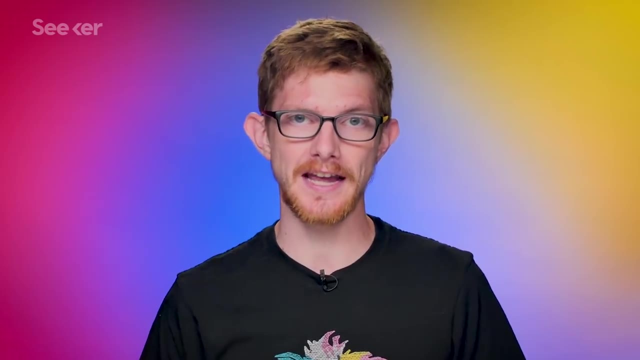 Prime numbers found this way, by raising two by a prime exponent and subtracting one, are called Mersenne primes, named for a 17th century French friar, hence the capital. M 3 is a Mersenne prime, since it's 2 to the second power minus 1.. Same for 7, which 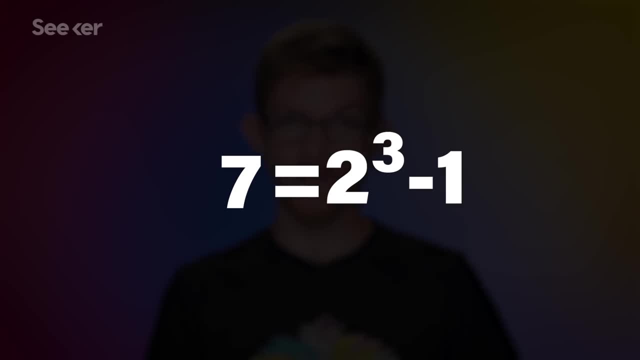 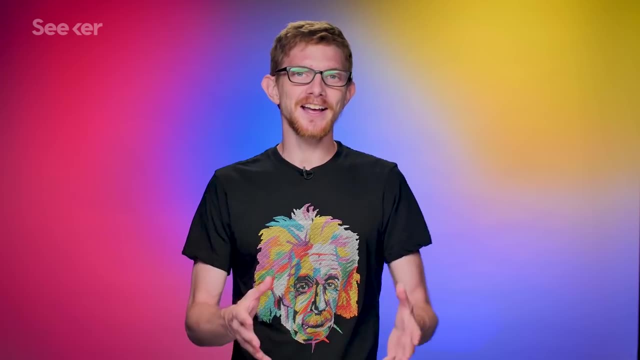 is 2 to the third power minus 1.. But the exponent has to be prime. 2 to the sixth power minus 1 is 63, which is divisible by 3, and so not a prime. Nine of the ten largest primes found to date are Mersenne primes, not because they're. 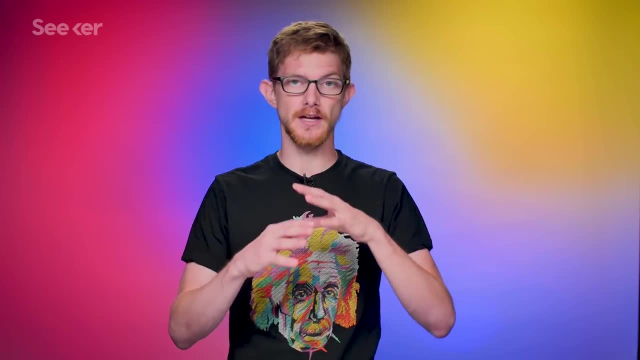 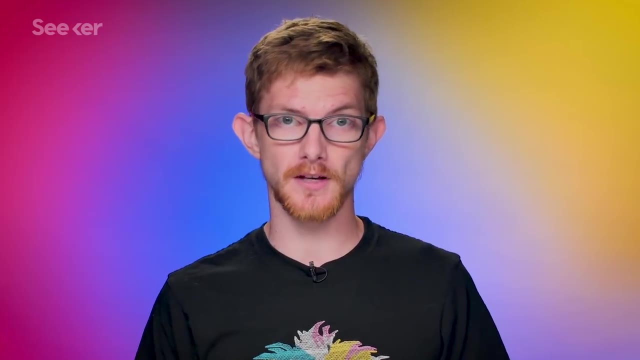 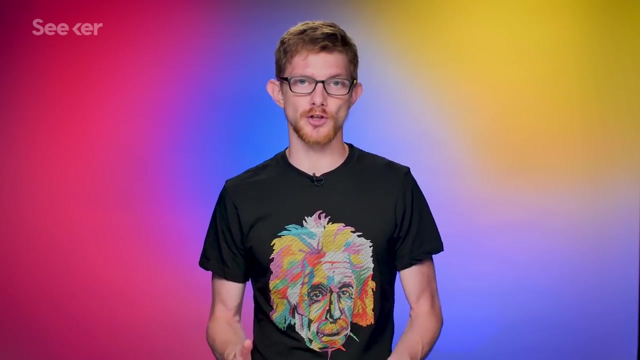 the most common. The prime number theorem tells us there must be a simply huge number of undiscovered primes between this newly found one and the first. But we find them this way because that's how we keep searching for them. In fact, you can be a part of the search for the next one. You don't even have to do the math yourself. 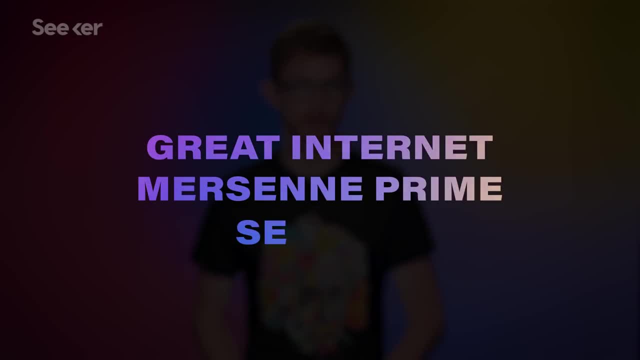 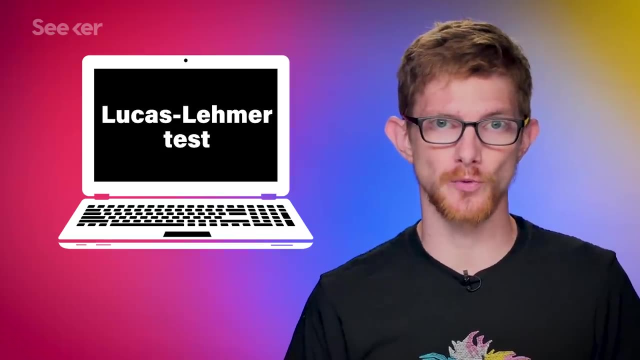 just some software provided by the Great Internet: Mersenne Prime Search or GIMPS. The software uses the idle processing power of your CPU to run what's called the Lucas Lemur test, where Mersenne numbers are checked against a specific set of numbers. If the 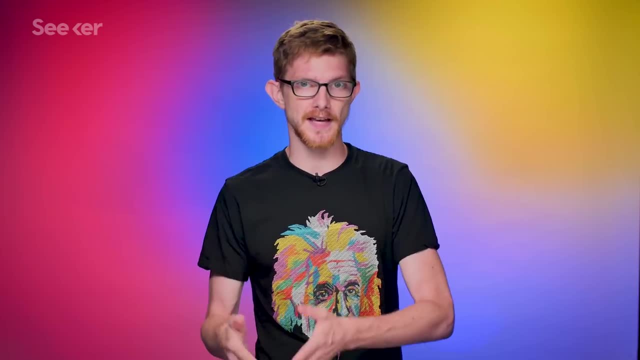 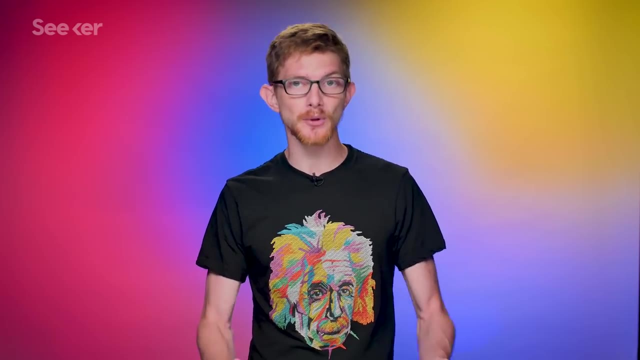 Mersenne number you're checking divides evenly into a certain number in that set, then it passes the test and is indeed a prime. Obviously, it takes quite a bit of horsepower to see if a 23 million digit number divides into an even bigger number, which is why the project needs the public's help. 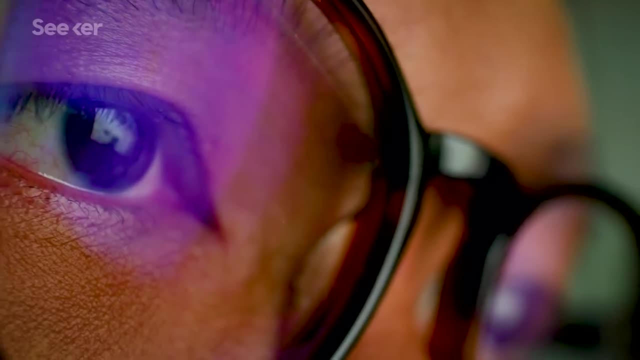 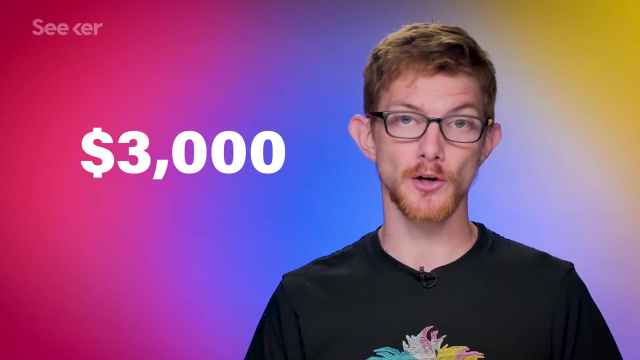 Almost 200,000 users are running the GIMPS software, and if their PC runs a number that passes the test, they could win money. Pace is eligible for a $3,000 prize, and whoever finds a 100 million digit prime could win $150,000. It's like cryptocurrency mining.